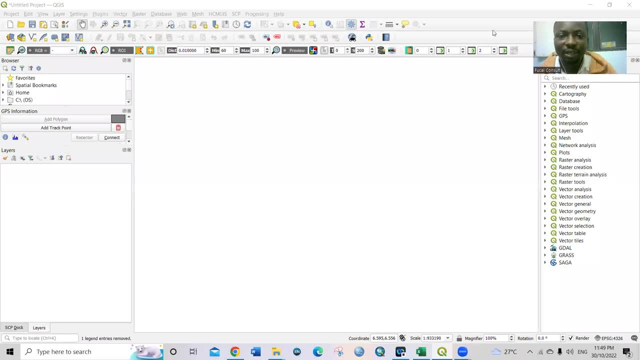 Good day everyone, from wherever you are watching this video. I'm presenting this video on how to perform a simple spatial analysis using QGIS. This is a very simple analysis of data which you can use QGIS to do. So if you're watching this channel for the first time, please kindly subscribe if you have not done so, so that you can encourage me to do more videos on this channel. 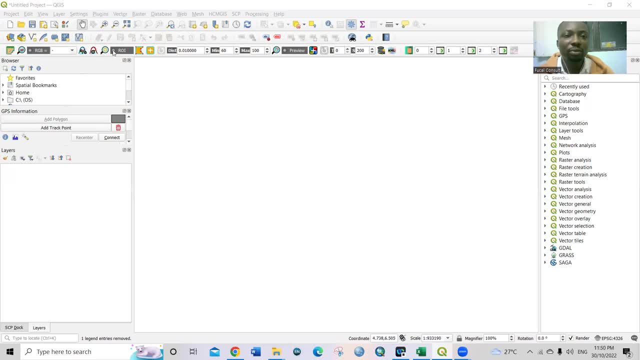 Thank you very much. So let's go straight to QGIS. So this is a QGIS software. I've already opened my software And I want to bring up a shapefile of a particular state, a country. So we're going to use this shapefile to demonstrate how you can show your data. 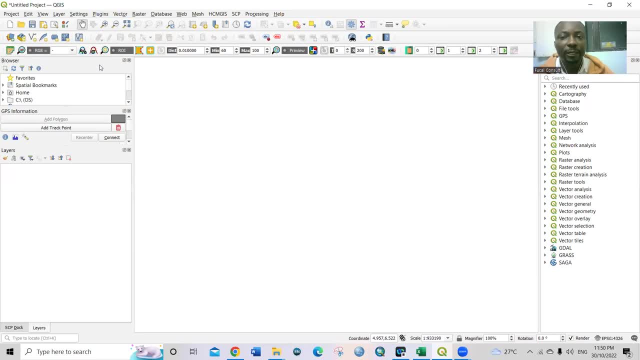 The data you know in form of colors, you know to represent each of the features that you are interested in on the map. So let me go to layer. Of course, it's telling me about how to bring up a shapefile, how to have a layer file in your map, your QGIS interface. 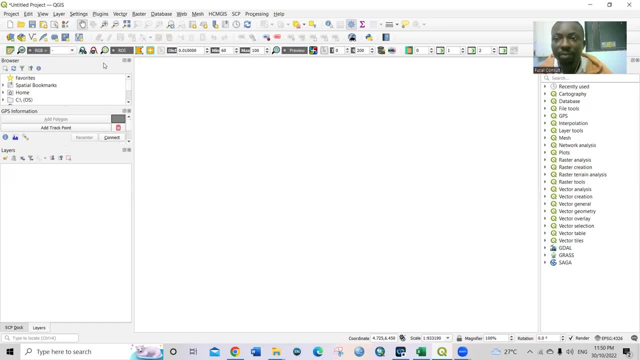 If you don't know how to do that, please kindly watch my previous videos on how to perform, how to do map using QGIS and how to extract file- I mean layers or shapefiles- from large country files. OK, so let's go to layer. Then you go to add layer. 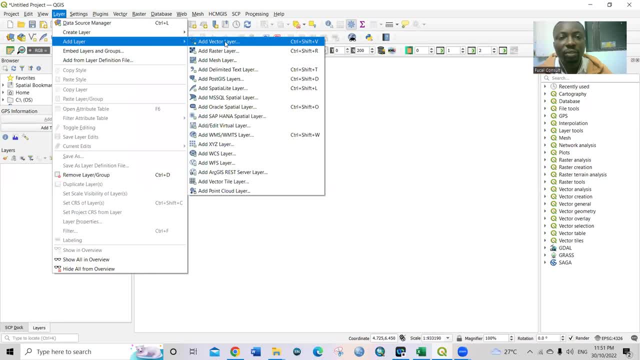 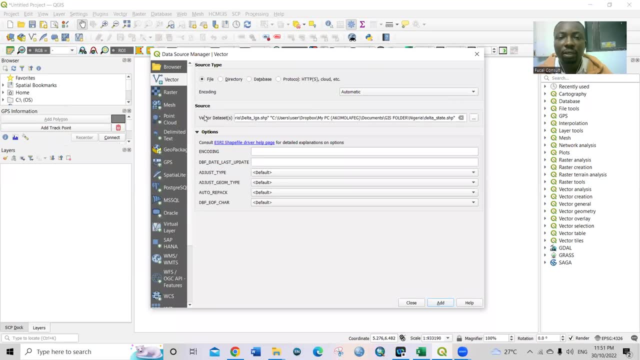 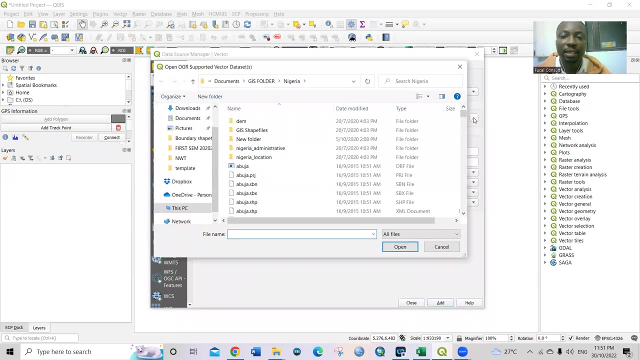 Add layer. Of course we're dealing with vector layer. So you click on add vector layer and this one will proper. Then you go to this and then browse to this And then browse to where you have the folder, The folder containing the country or the state or the district that you are interested in. 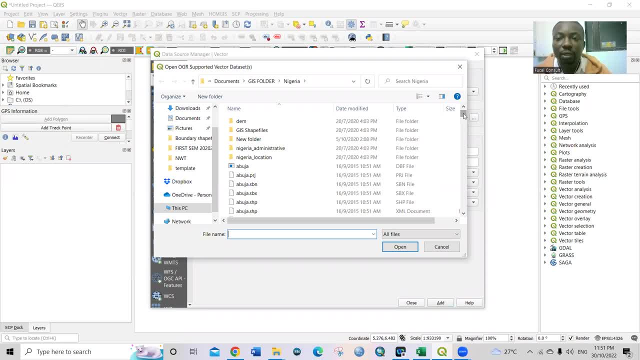 that you want to, you know, do a spatial data analysis on. So let's go to the one that I'm working with. OK, so I'm going to bring up a particular state with the districts Or the local government areas in the state. 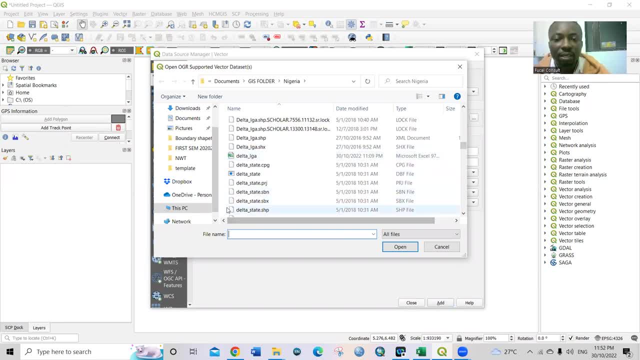 So I'm going to click on this data state. Data state. I want to pick two shapefiles, So I'm going to press my control key on the keyboard and then move to select the second shapefile. So I'm working with this one also. 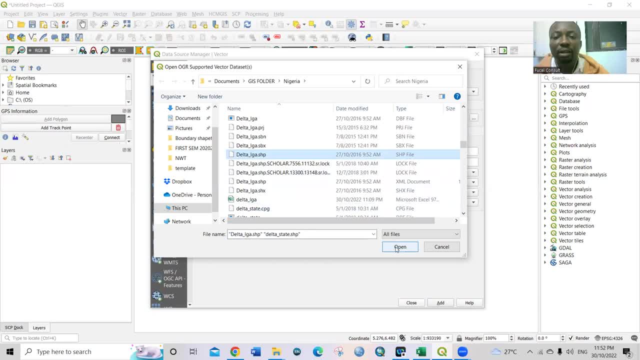 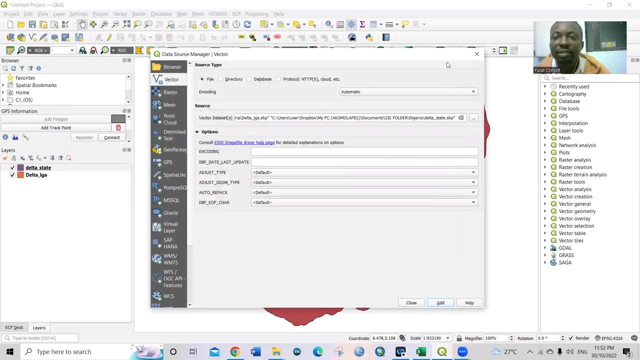 Delta LGA shapefile. So then you click open. After you click open, then you click add- All right, And then QGIS has automatically added the shapefile as a layer for you to work on. So I can close this one now. 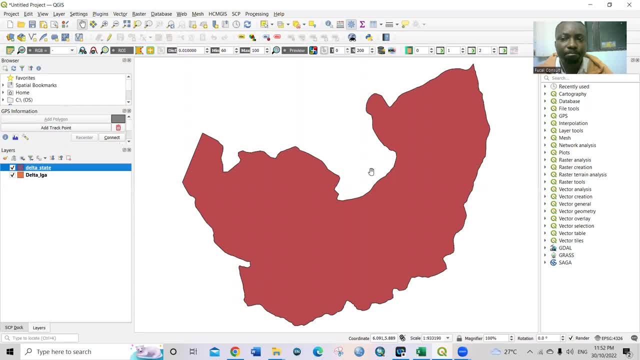 Just click close. Now this is the state. There are two different layers that I brought up, Or two different shapefiles. The first one is the state, Then the second one is the local government areas, or in some countries you might call them districts. 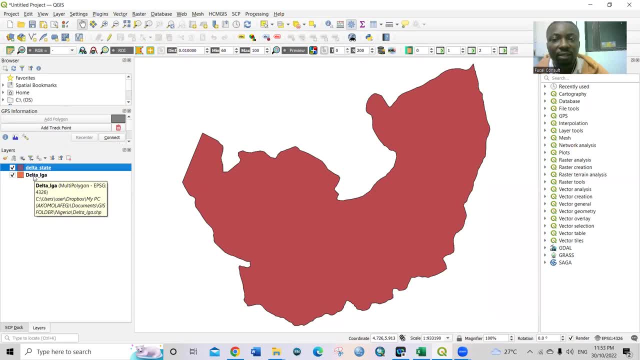 Districts in the states. So now, if you uncheck this one, you'll see the district will come up like this: So this is the district And then inside the district there are different- sorry, inside the state there are different data that have been used to, you know, to bring up the state. 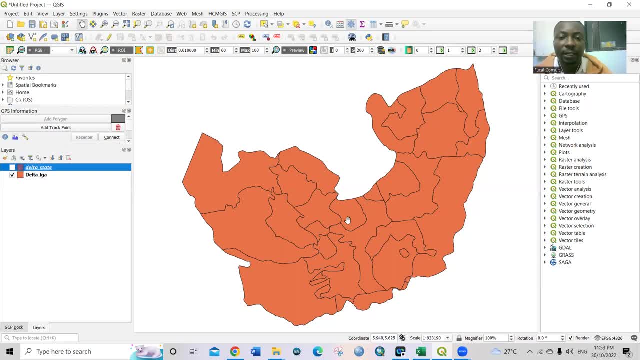 You know, to bring up these particular local government areas or districts So for us to be able to view the data. you right click on this Delta LGA. Right click on it And then go to- if you remember you know- previous videos. go to open attribute table. 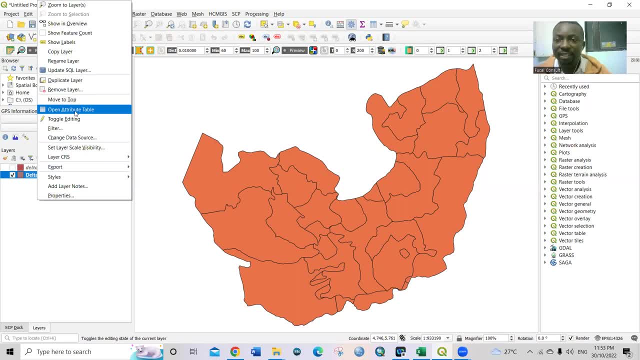 So open attribute table will show you all the relevant data That are already you know in this shapefile, That have been saved or stored in this shapefile, So you can manipulate those data as you wish. So let's click open attribute table. 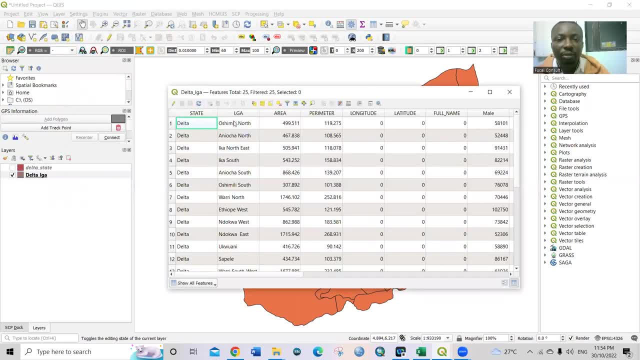 Now open attribute table. you can see now it has come up. You can see: this is the Delta state, This is the local government area or the districts. Then these are the different data that have been used or that have been stored in this shapefile. 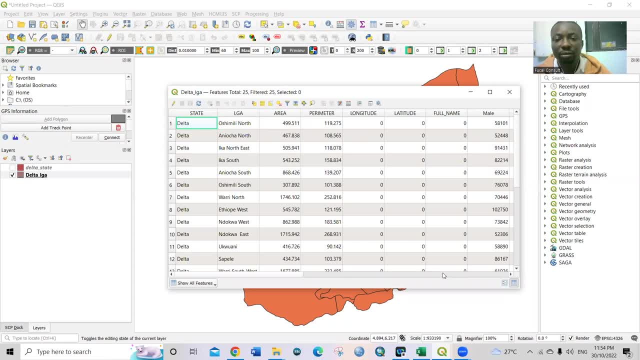 Which we can. it can give us Different kind of information on each of these local government areas. For example, look at this area. This is the area of land, This is the perimeter of land, This is the longitude, latitude. Okay, these ones are empty. 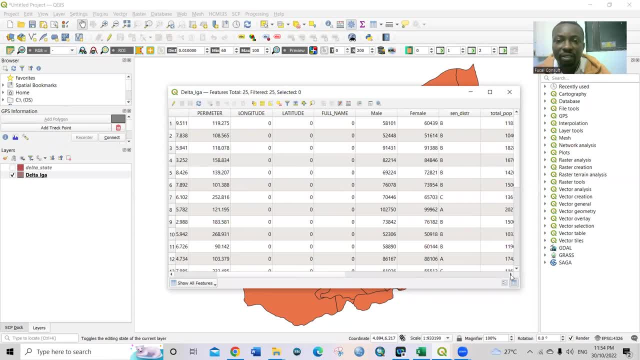 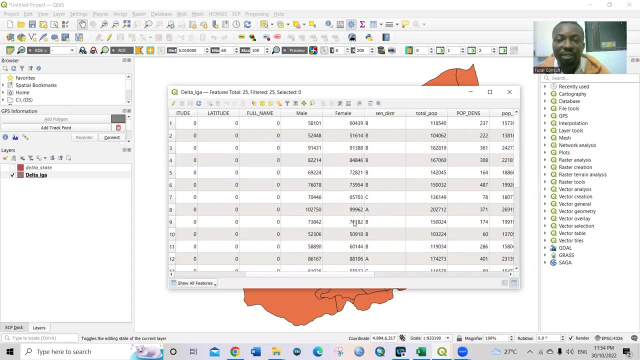 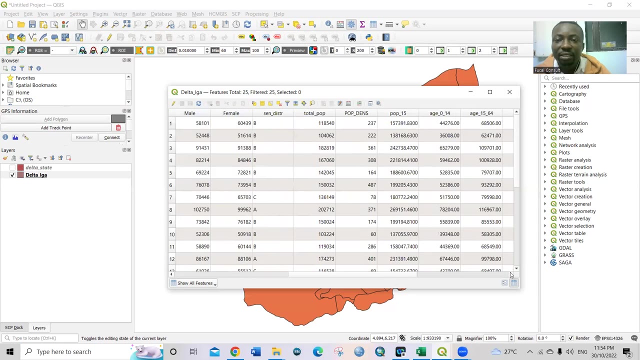 They can be filled in later. So let's scroll down, I mean to the other side. You see the number of males in each district. See the number of females in each district And then see the total population. All right, See the different data there also. 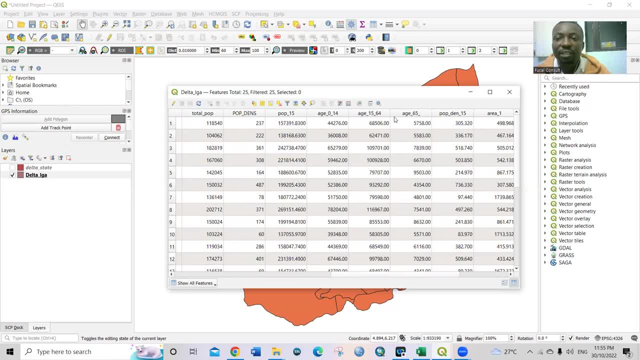 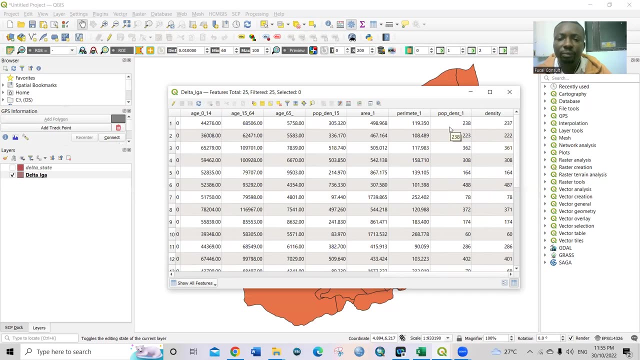 Population density. See the different age groups: Age 0 to 14.. Age 15 to 64. Age 65. You know different age groups And then the other data also there. So now let's assume that we want to work with the land area. 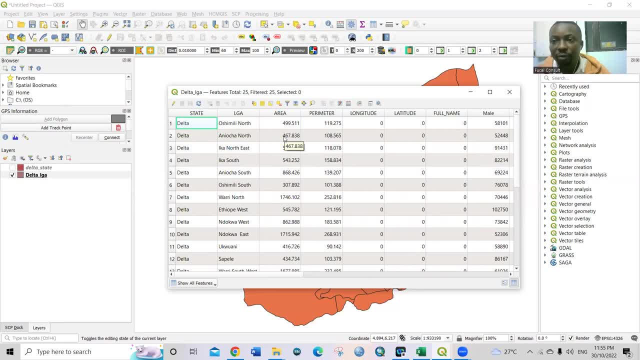 The area of land. We want to show on the map The distribution of the area of land. All right, You can also pick any other data that you are interested in. You want to show the number of males Or how the males are distributed in each of the districts of the states? 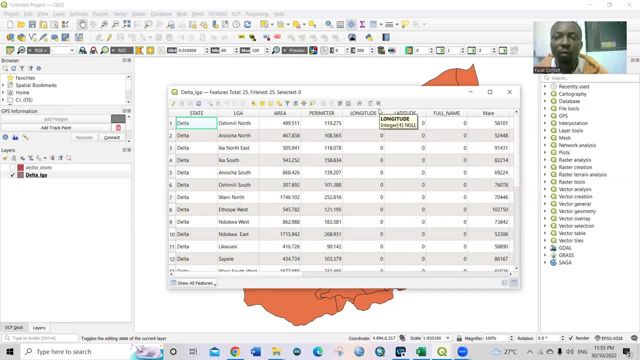 Now I need to say that if you are working with another thing, then that is the same principle. For example, maybe you collected your sample from different places. like I taught in my previous videos, If you're working on a particular area, 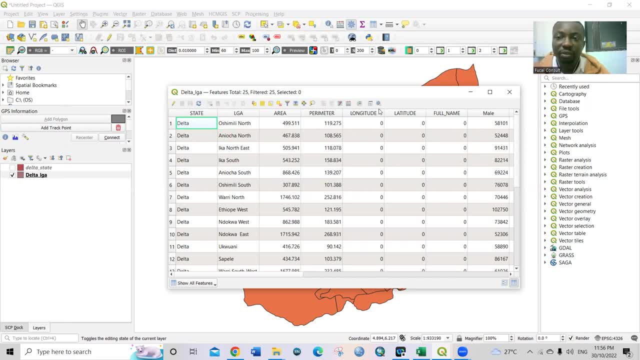 and then you collected samples from those areas. You can also use the same principle to show the number of the plants or animals, or number of questionnaires or whatever you collected in each of those sampling points. All you need to do is to bring the data up in this. 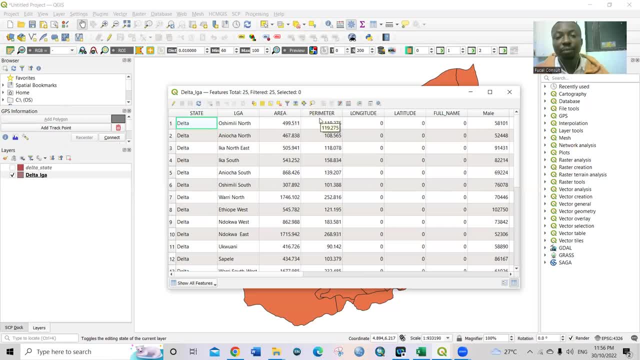 you know attribute table. Now let me quickly show how to do that. If you do not have, for example, maybe you let's assume that this area is not there And you want to put in the area of land or the area of 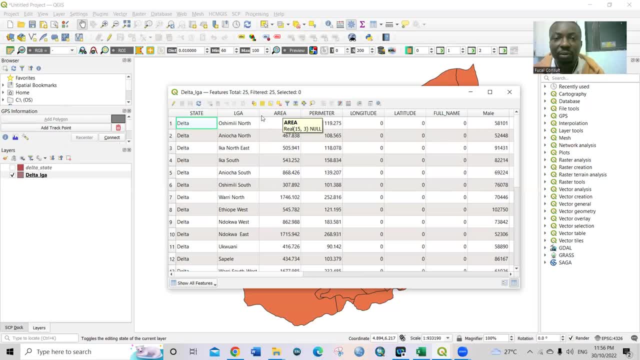 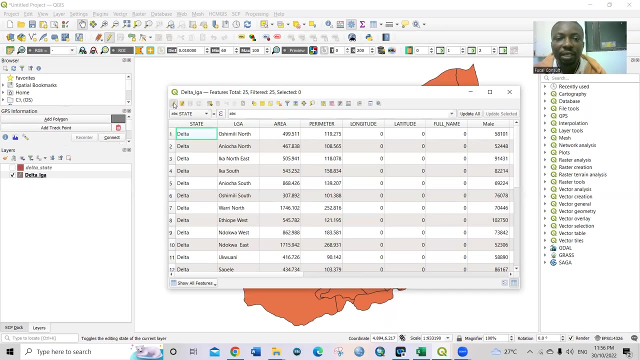 or any parameter you want to put in this attribute table of this shape file. What you would do? simply go to this, the left side of this window, you see what you call toggle editing. Click on toggle editing. Once you click on it. 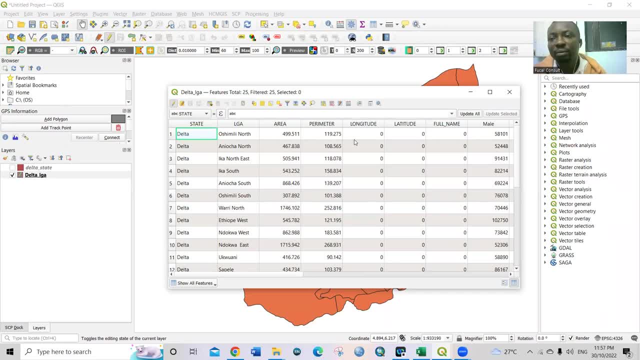 that means what? that means that you want to edit this table. You want to add some features, You want to add some data into it. So after you click on toggle editing, then just move your cursor to this side. You see, then this one tells you: add. 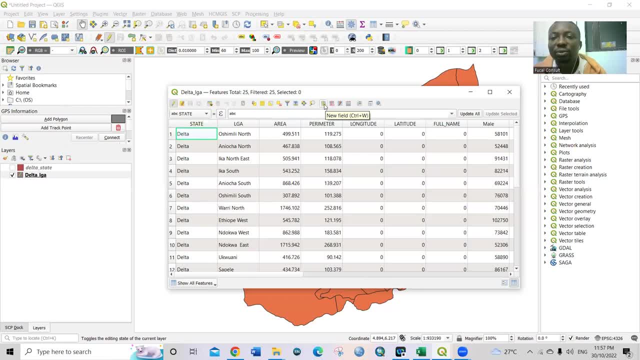 it's a new field. That means you want to add new column, You want to add new feature to this, to this table. So just click on new field, Then this one will come up. Then you can give it a name. Let's assume that we want to put the area of land is not there before. 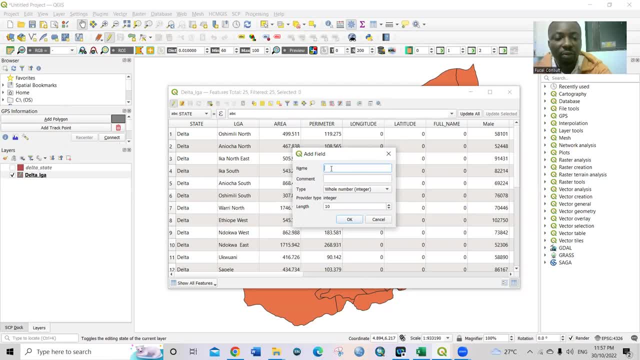 Don't forget, you can use anything, You can input any data. So I want to put area, All right, So area. then it asks you what type. you can leave this one blank, Then this one. you say what type. 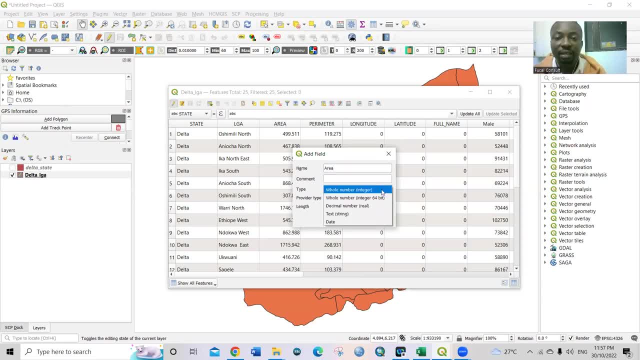 what is the type of the data that you want to add? Is it a whole number? Is it a decimal number? Is it texts that you want to have? Is it dates you want to add? Now, in this case, we're adding area. 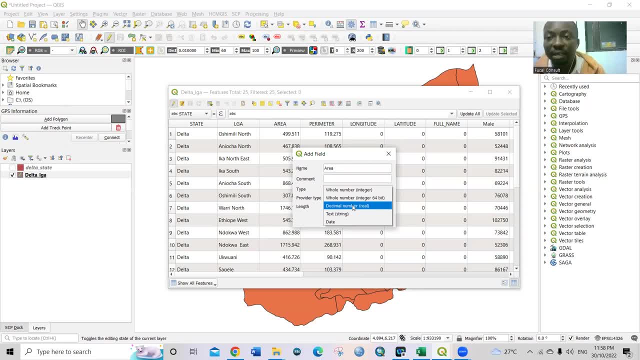 Area of land can be decimal, can be decimal a unit, So just click decimal. When it asks it tells I mean it's asking you how many length or the length of the units, So just leave it at 10.. Sometimes you might have area of land that is up like 10 digits. 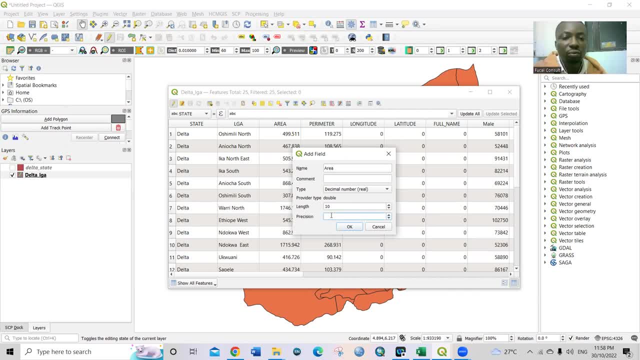 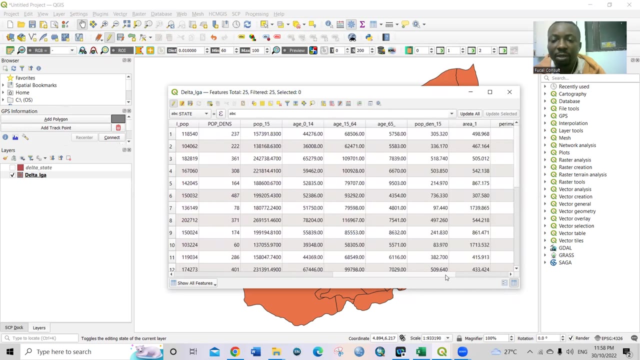 And then precision. you can leave this one as two, you know, and then click OK. Once you click OK, the column would have been created in this table. So let's scroll down, I mean to the other side, and see whether the column has been created. 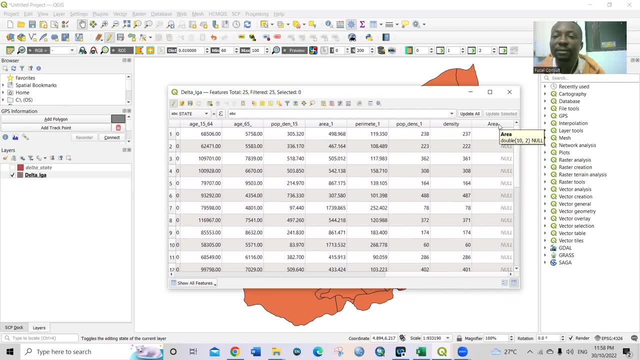 You see, now the new column has been created. All right, So all you need to do now is to put in the values for each district inside each of this row. Each row represent each district, but you have to be sure which one you are having. 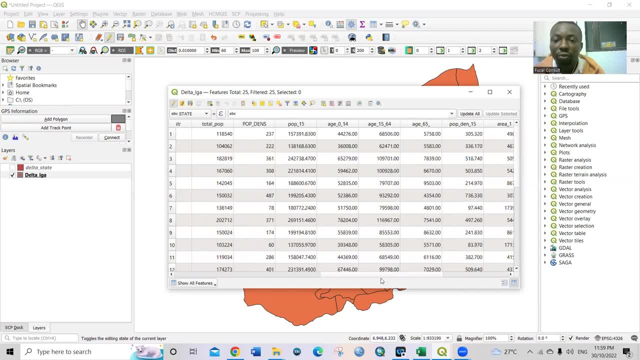 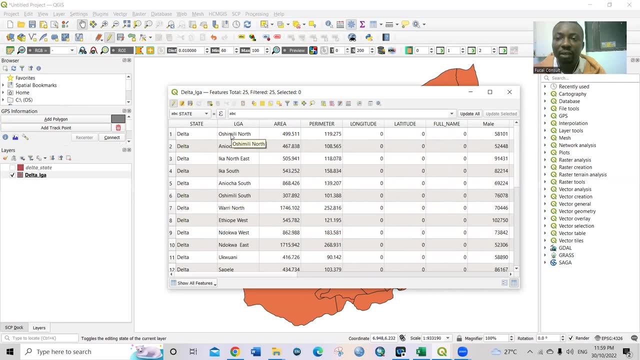 So if you are having this first row, you need to know. scroll to this side to know what's the name of the. okay, the name of the loop government is this, So you can check in your record and then get the value for this particular district or local government area. 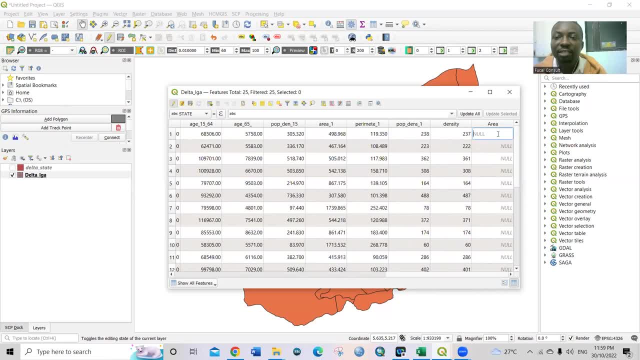 and then come to this side and click inside this place and then type. you can type the figure, Let's say 64, 645.65.. Right, You see, now it's there, So you can put the second one. 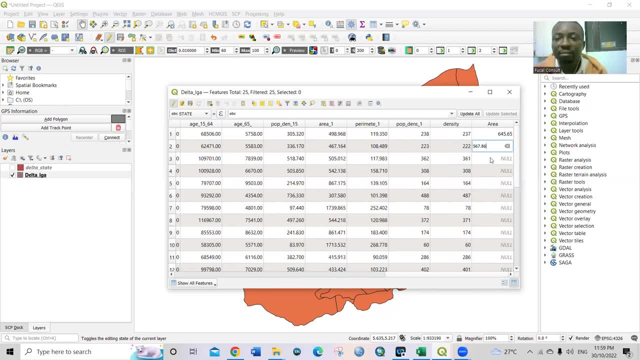 56, 7.86.. It's there So you can add all the area of land, all the data. you can add it down until the last one And when you are, when you are done with inputting this data. 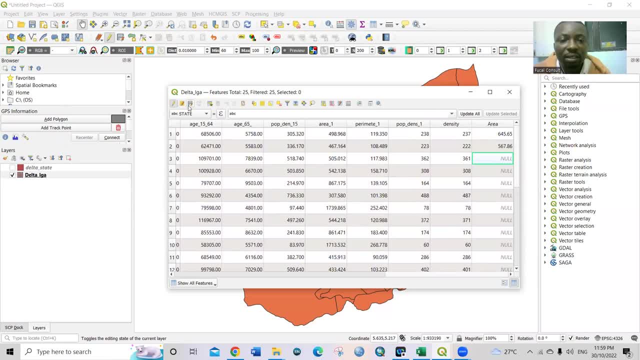 just go back to this, these icons here- and you see save edit. So you just click save edit. Once you save it, the data is permanent, Just like all the other ones that have been saved already. So it's permanent. 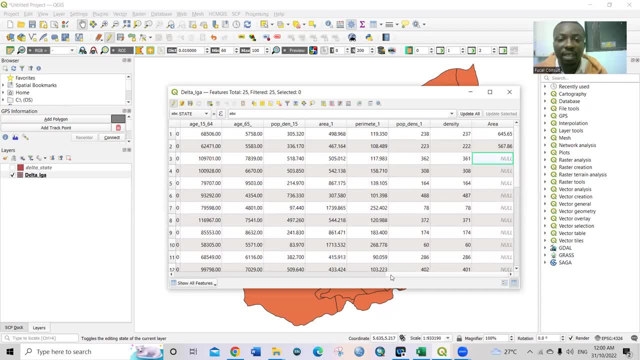 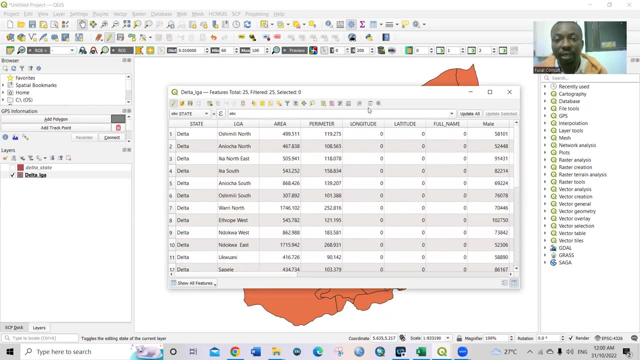 So, but because we already have this area as part of the shape file, so I don't need to create any other data for area of land. If there is another feature, I could do that, So, but now I'm working with area of land. 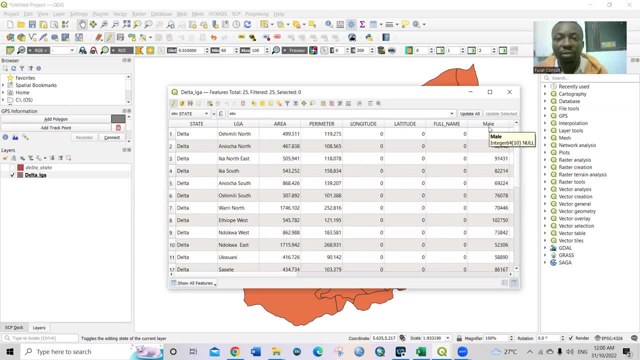 I want to show the area of land on the map. So what I will do is just to ignore the other ones. So I just close this, Just deselect this. Then it's asking me: do you want to save the changes to layer depth? 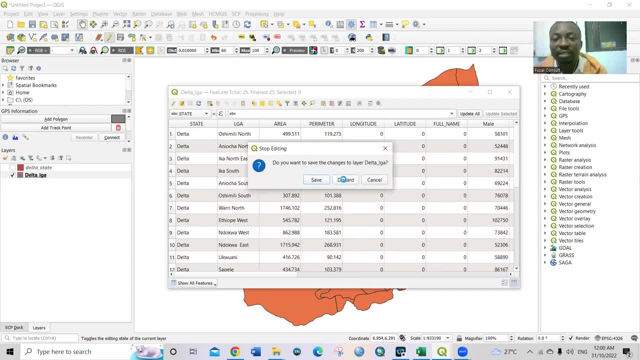 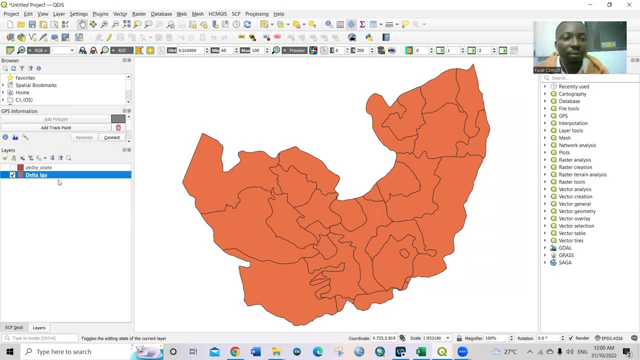 So I say no, If you want to save it, you can click save, but I say discard. All right, so it's discarded already. Then I close this, Then come back to your this map here. So what you would do now. 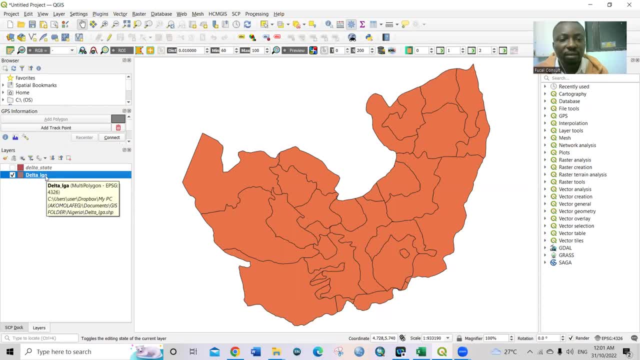 is to simply right click on this on the table of content, right click on the, the data LGA, And then, after you right click, then go to properties, go to properties, right So, properties. we want to put a label on the. 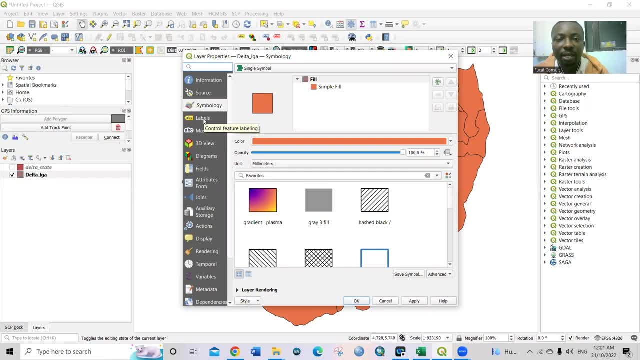 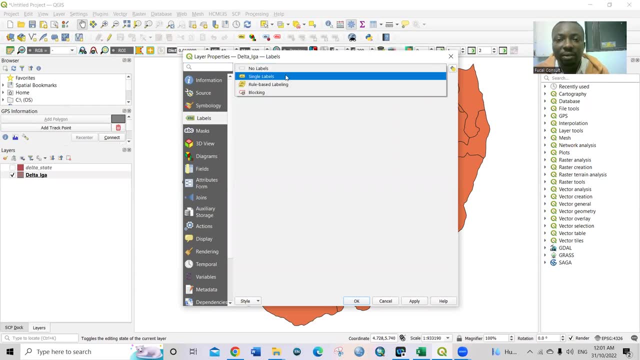 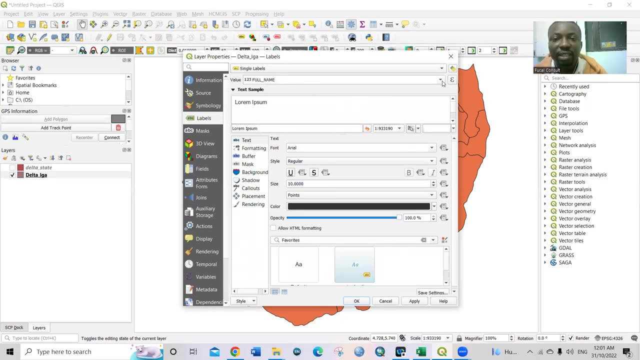 on the map. So click on label and see label here. Click on label, then come here. it's telling you no label. So you just select it and click single label. So once you click single label, then you now select, then you now select which of the column you want to. 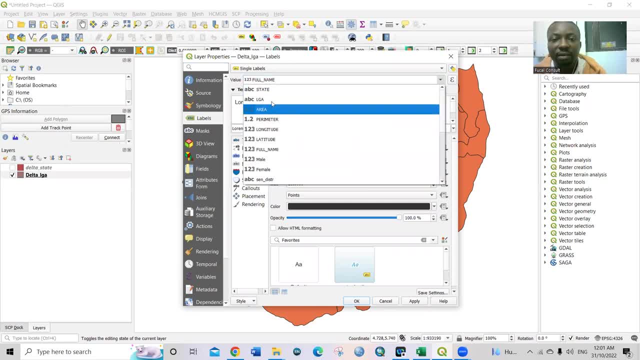 you want the name to appear on the map, So normally is the- is a local government area because the state- all of them have the same name as state or different names as local government or district, So we're going to select this one. 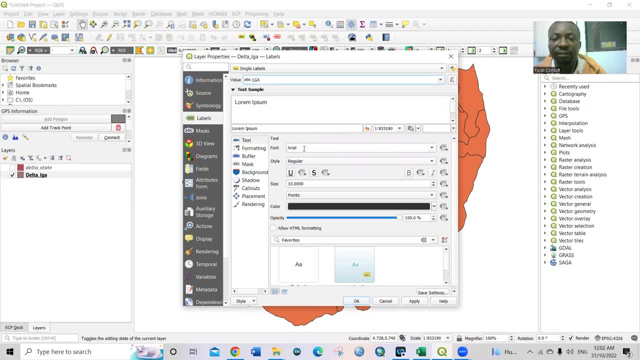 local government area, Then you can. you can select the font size you want. You can select the. you know the style. You can select the size of the font. You want it bigger or smaller. Let me just increase it to like 12 or 13.. 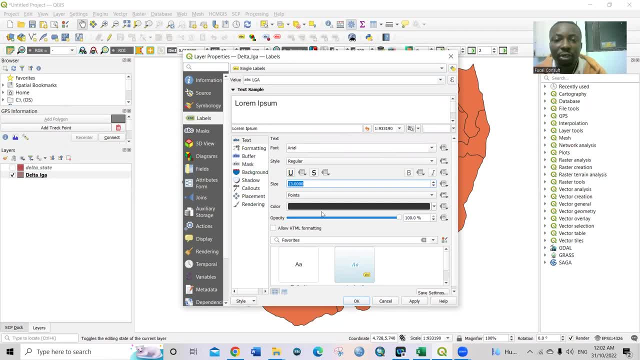 Yes, Okay, Then when you're done, just click All right, I want to also change the color. Okay, Let's just take the color for now, because the color will simply change later on. So let's click apply and see what we have done. 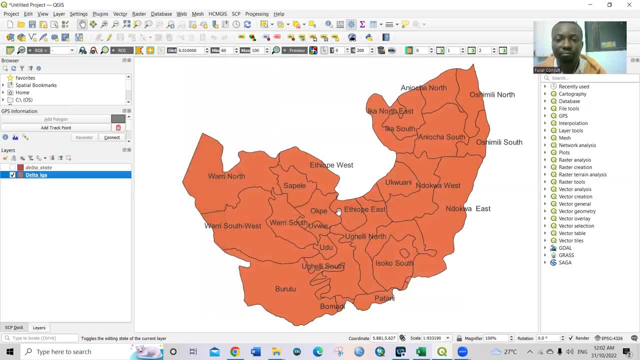 Okay, All right, You can see the. the names are already there. The names are there. You can see the names of each, each local government areas of the states. Now let's go quickly to what to now show the distribution of the land areas in form of colors. 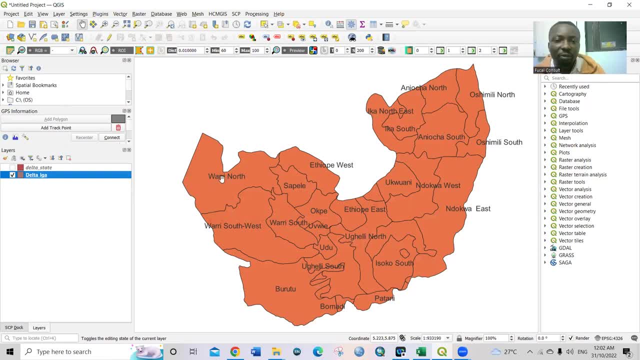 So that whenever you look at the map you can know which part of the local government has. you know, so, so, so, range of land areas, which one is biggest, which one is the smallest in terms of. so we can show that with the color. 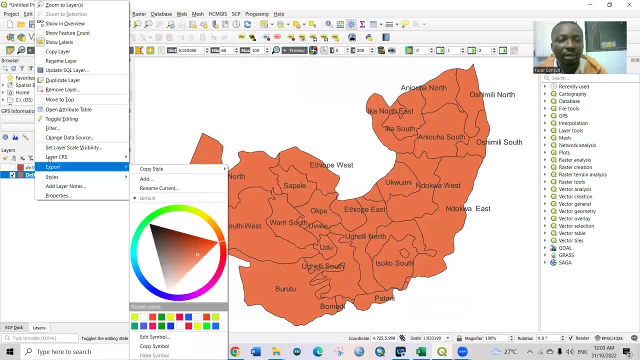 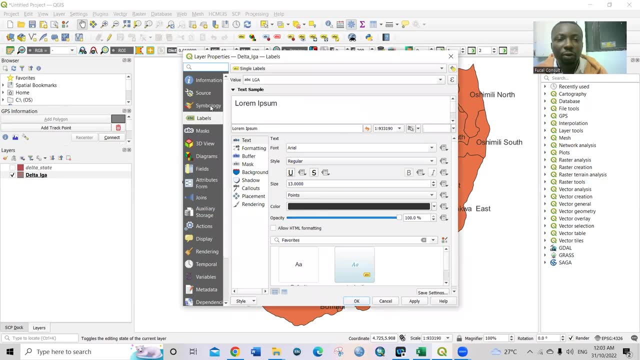 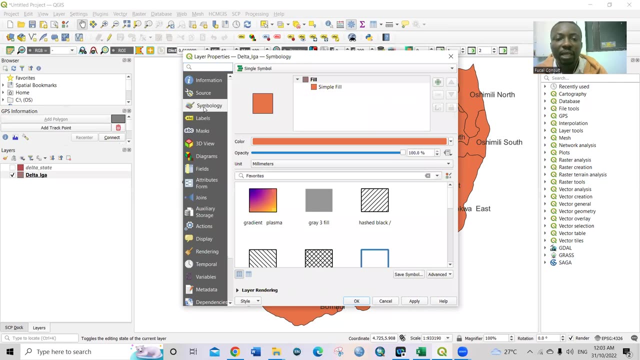 So let's go back to right click on the Delta local domain area, Go back to properties, Then go to what you call symbology- Symbology just above the area, or above the label, rather. So go to symbology Now under symbology. 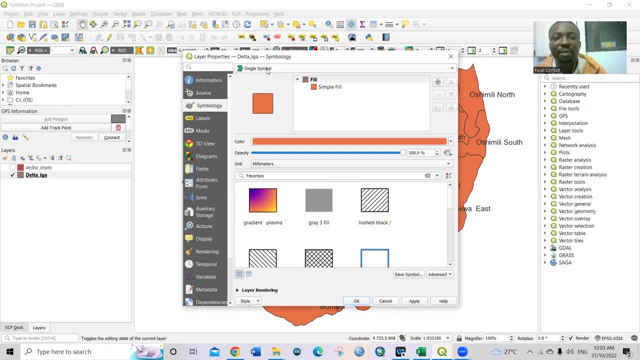 the first thing here is telling you: single symbol, because all of them have the same color. Well, you want to show different colors in terms of the area of land, So we have to click. come here and click what you call graduated, Just click graduated. 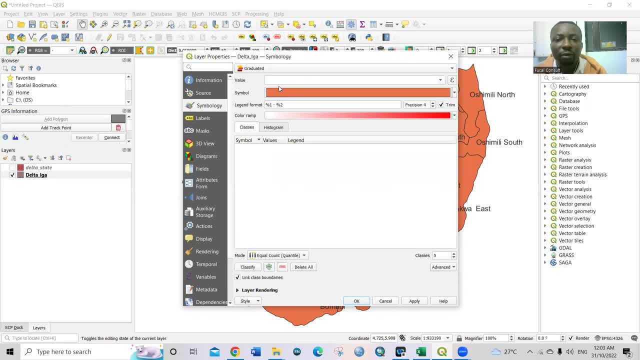 Graduated Right, So we've already clicked graduated. Then let's come back here now to select the range of colors that we want. Range of colors, The color ramp: How do you want the color to be So just like the range of color? 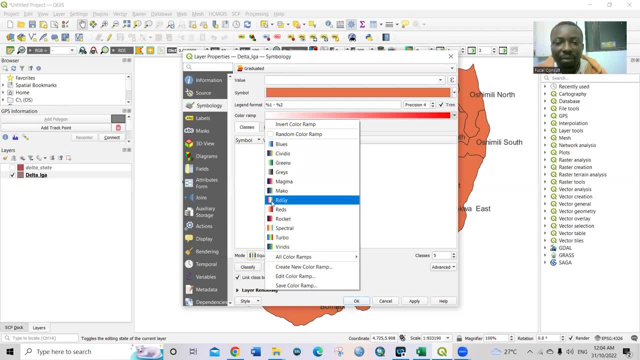 So and select different types of color based on your choice. Let me select this one, Let's see. Okay, All right, So let me select this. This one is red to like blue or so Okay, So I haven't done this. 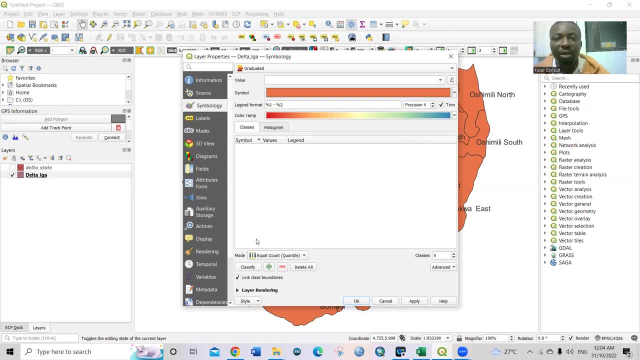 The next thing to do is not to bring up the areas, The area of land. So then you come here and click classify, Click classify, Okay, Okay. So you click classify And then, after you click classify, the next thing is after you click. 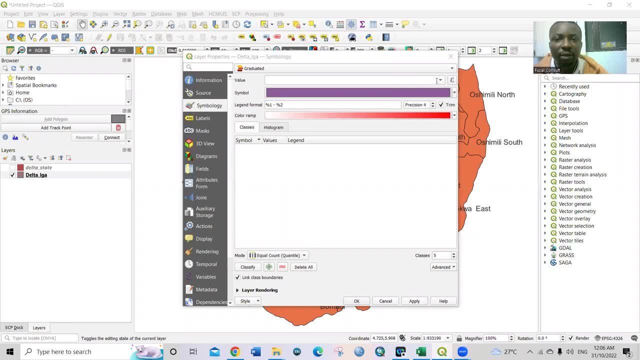 uh, classify. uh, you need to. uh, we also have changed this value After we selected this as graduated, we also have changed this one to uh, what to call? So click on this value so that we can select which. 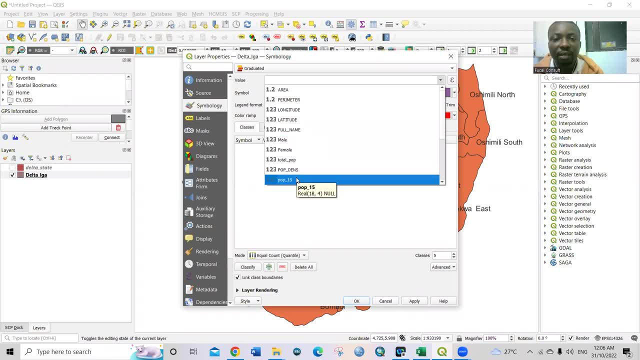 uh data. we want to represent uh on the map. Is it area? Is it perimeter? Is it different? No, So, but because we want, we're interested in the area, So click on area. So after I click on here, 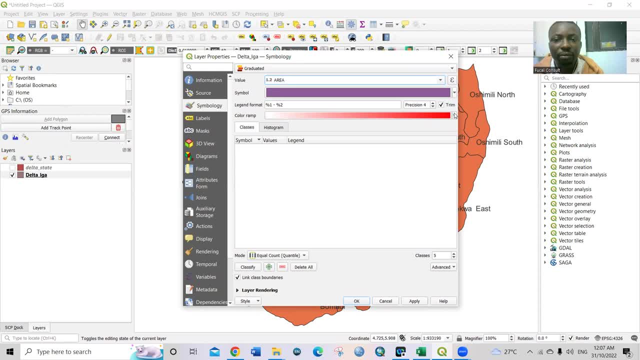 uh, then okay, we need to. this color ramp is um. which one did we choose? Um, okay, You can select any color based on your choice. All right, So now, uh, so just click after you select this area and you click classify. 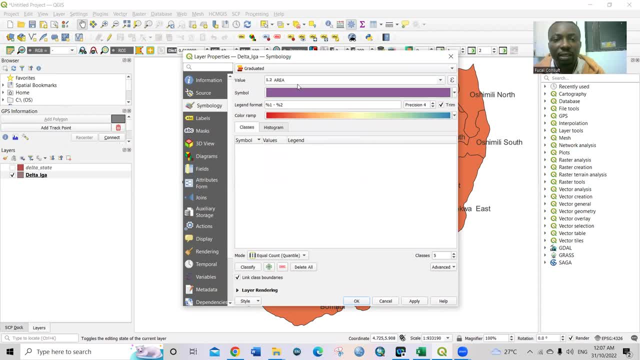 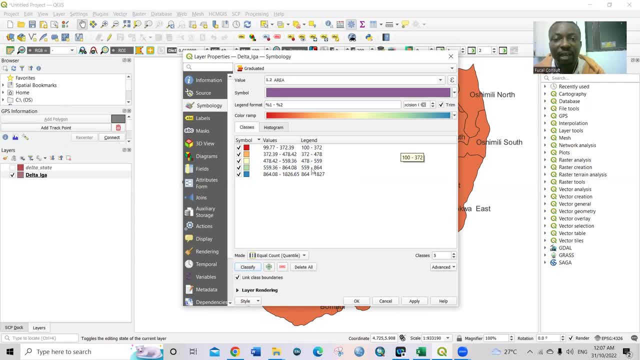 in the in the in this uh shapefile, the QGIS has been able to classify the areas of land from the smallest to the highest, And it has given each of them a range of values. So you have between 100 to 372 square. 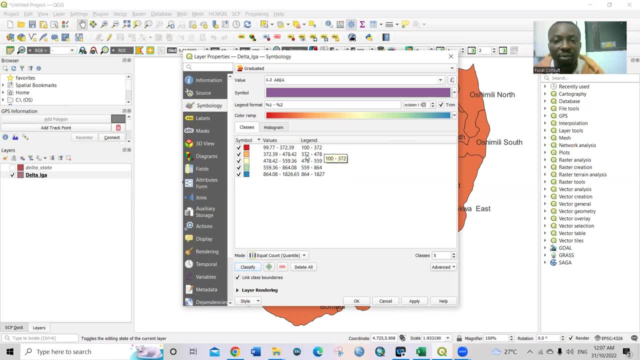 uh square meters. Uh, then you have within 372 to 478.. So you have each of them, uh, like this, So, and each of them has different color representing uh them. So by, can we? so? do you want it to be more than five classes? 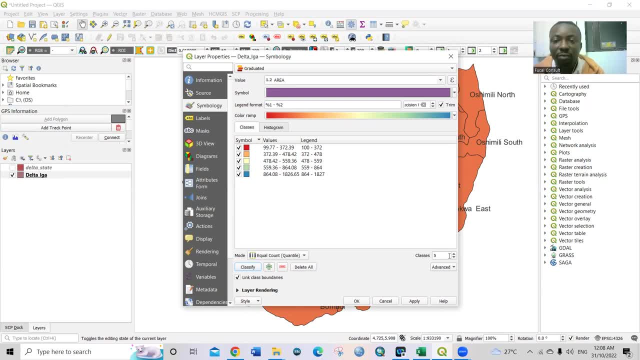 Because these are just five classes. If you want it more than five classes, you can come here and select: uh, six classes. You can see it has already given us six classes. Depending on the number of classes, you can make it more than six or seven. 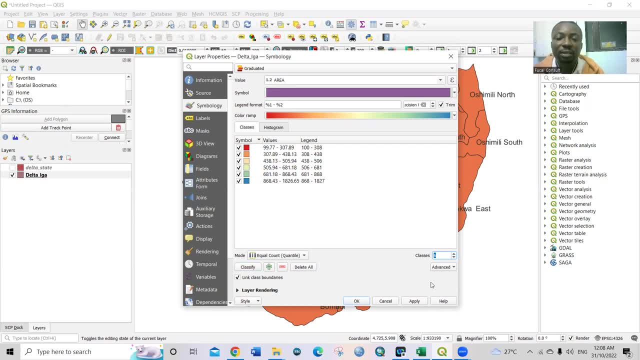 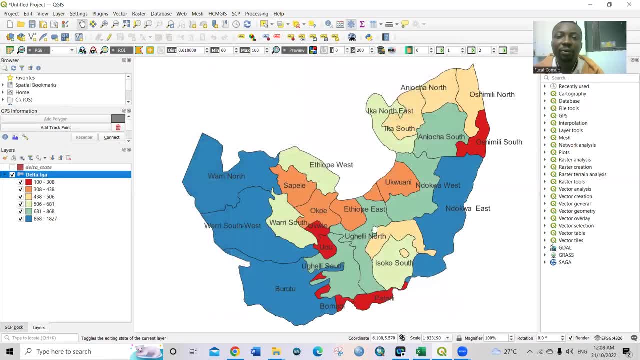 I don't click. Okay, Now you can see from the map you guys as been able to uh show us uh the different classes. Look at the table of contents so that you can know which color represents which uh. 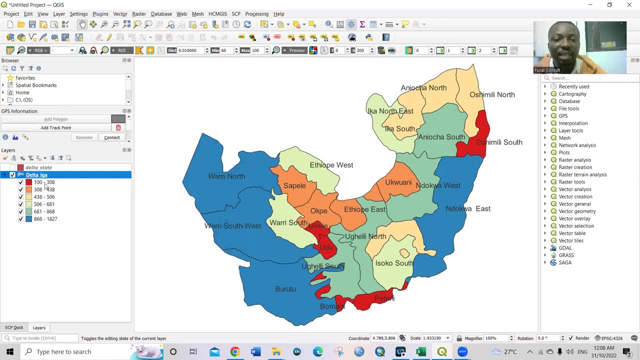 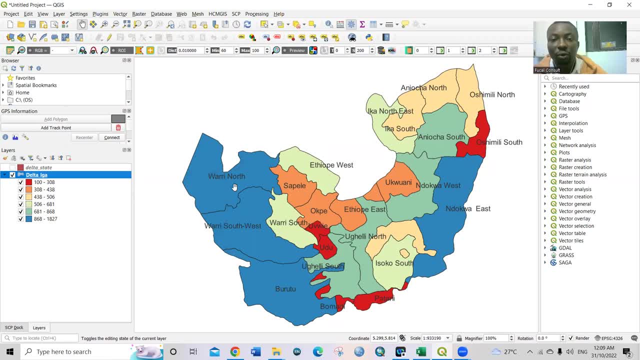 terms of the land area in the state. so that is uh, uh, how to show your, uh, how to show the, the, the area or a particular data. don't forget, i said you can use any data to represent, uh, to do the spatial analysis. it's not, we just use this area to show on the map and you can see the areas. 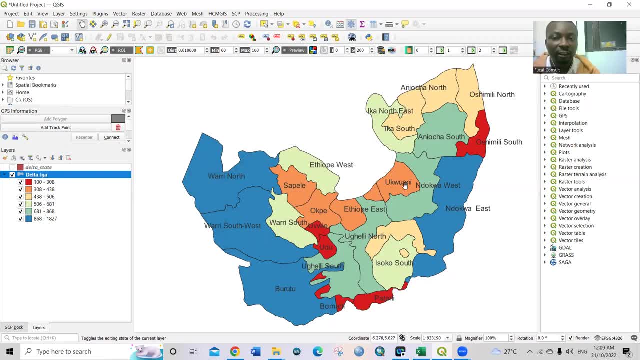 of land, uh based on different colors, have been shown on the map. any data at all you can do with this uh, you know, with this type of analysis, and then anyone that looks at your map will know the range of each of these uh features that uh you are working on. all right, so this is how to do this. 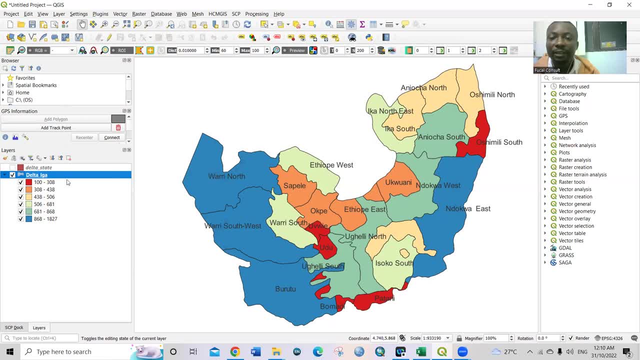 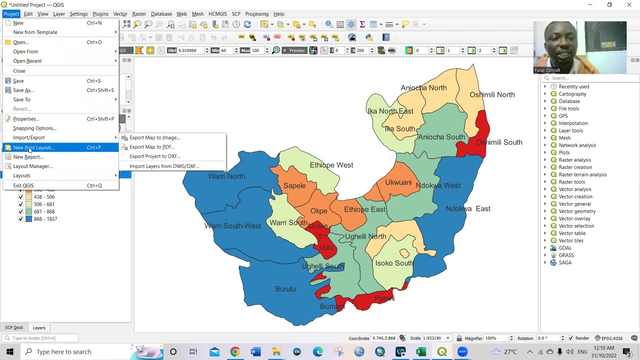 uh, if you now want to do the- uh, the final design of the map- i already thought you had to do that in my other video. uh, let me just quickly give a brief- uh, you know- summary of that, so just go to projects. click on, uh, new print layout, because keep guys has two different layouts. new print. 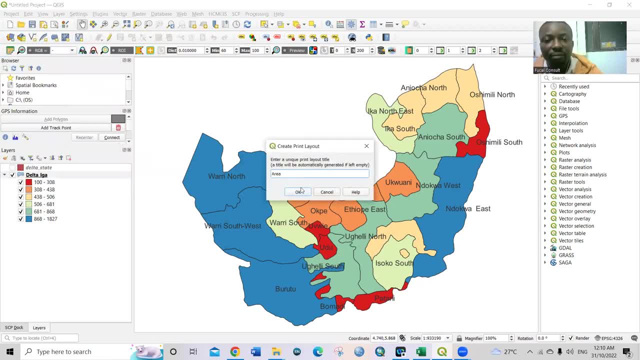 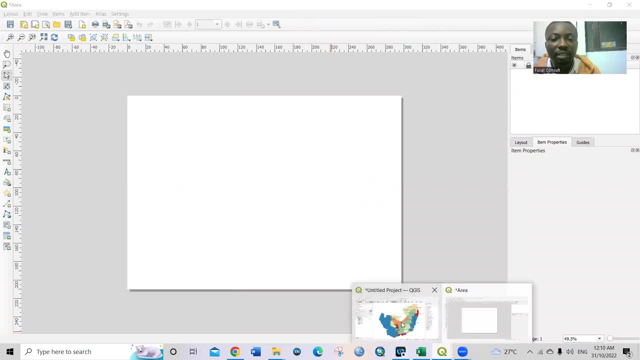 layer, so give it a name. i'll say area and click ok, then the print uh layout will come out. and then, because you have already uh, let me go back here, because i've already selected this map. anything you do you draw on this print layout will be the map that you have selected. 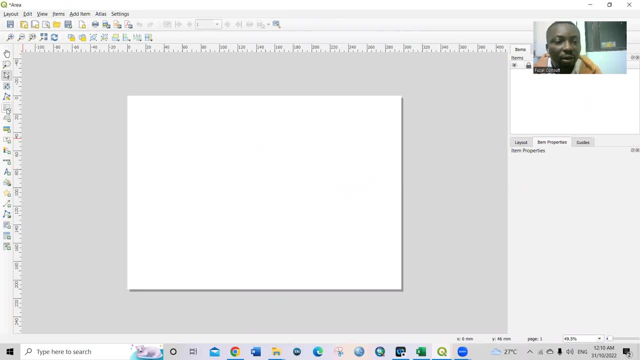 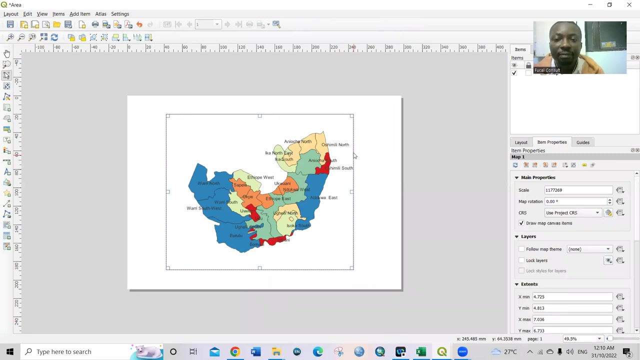 there in the other data layout. so just click. come to the left hand side and show add map. click on this add map and drag it here. drag it here right, so your map is there. then you can do the other, uh, other manipulation from this item property by the right hand side. 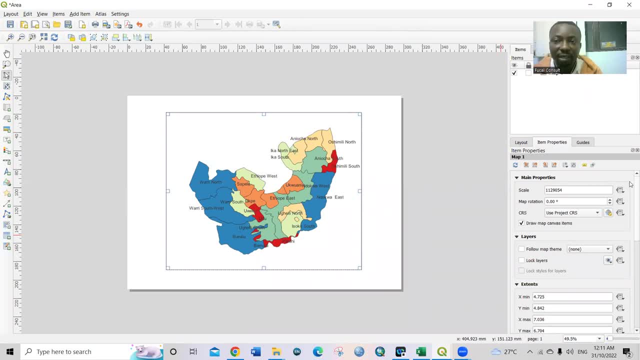 i will not go into the details today because you can watch my first video, or the, the video i did on how to produce third area map using qgis. just the later part of the video will tell you how to input all the map element: the legend, the uh, the arrow, the arrow uh symbol, i mean.